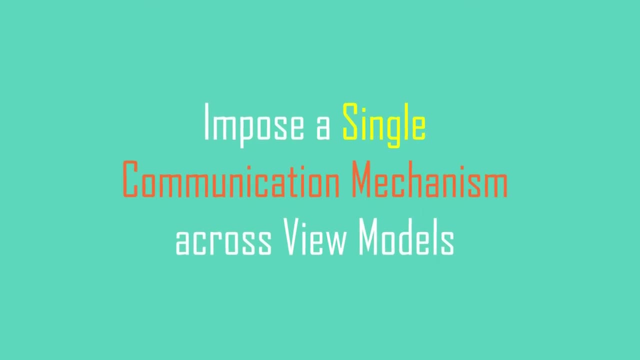 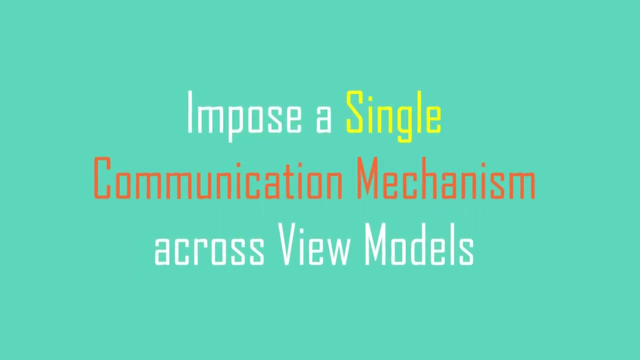 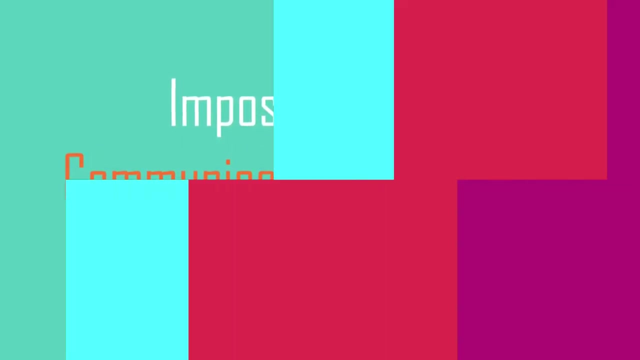 to someone else and impose a single communication mechanism across view models. That way, code maintenance becomes easy as well as definitely it will reduce system bugs, because generally most of the bugs are injected during the interactions between objects. We will understand this by working on a simple console application as well, as we will see. 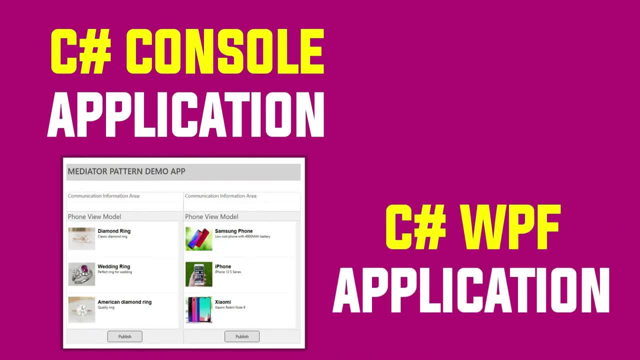 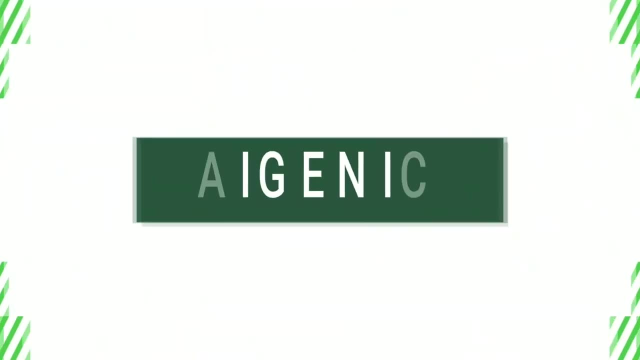 how this pattern can be implemented in a generic way in a real-time WPF MVVM application. But before that, make sure to subscribe the channel for all the future videos on C-Sharp and other NET technologies. With this let's get started. 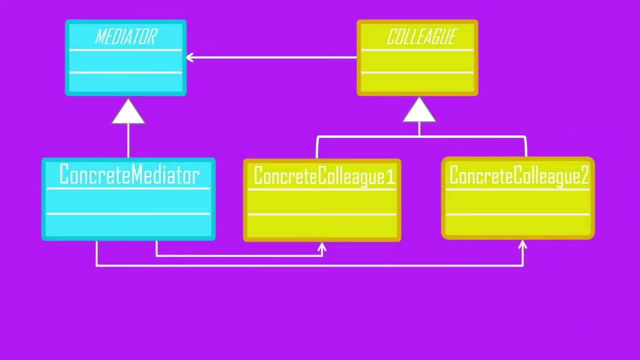 So this is Mediator Pattern UML. The naming conventions are as follows. I would like to change it a bit. Let's make the Colleague as ISubscriber and Concrete Colleague 1 and 2 as Subscriber 1 and Subscriber 2.. 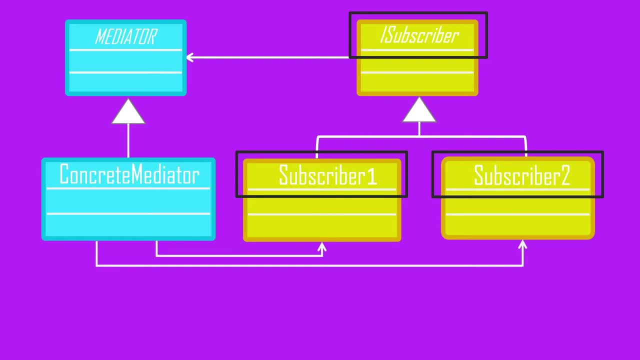 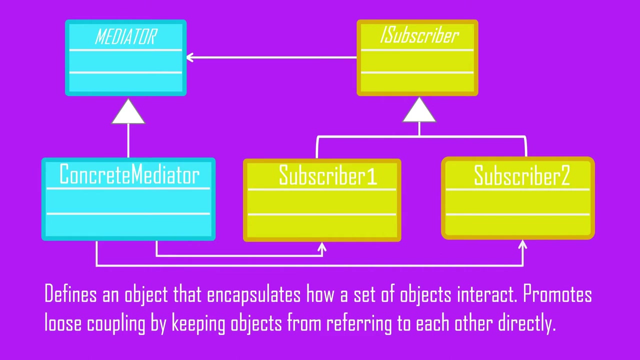 Don't worry, we will discuss about each component in a bit and I will ensure that by end of this video you will be able to implement it in your real-time projects. Let's see the definition once. Defines an object that encapsulates how a set of objects interact. promotes loose coupling. 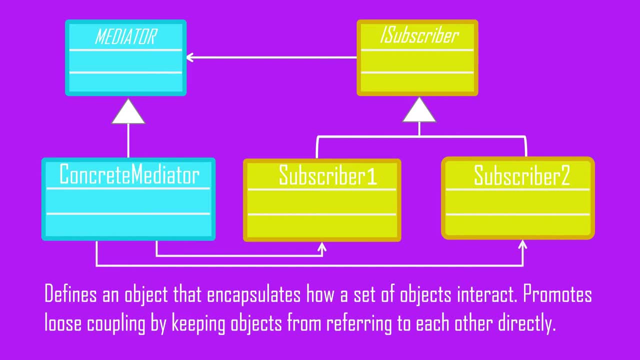 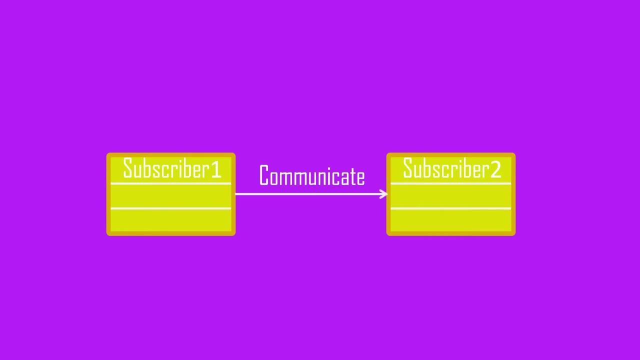 by keeping the objects from referring to each other directly. In short, Mediator Pattern encapsulates how objects communicate with each other without referring to each other directly. Let's break this down and understand. Say you have two classes, that wants to communicate with each other? 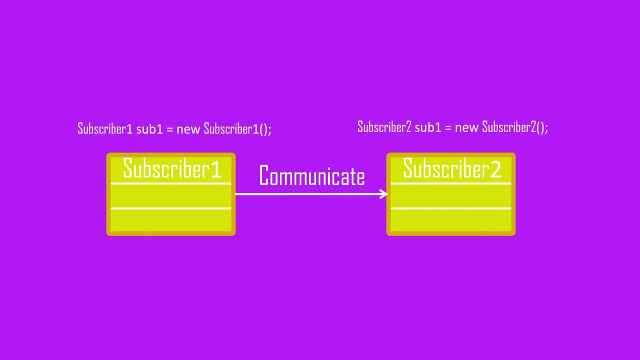 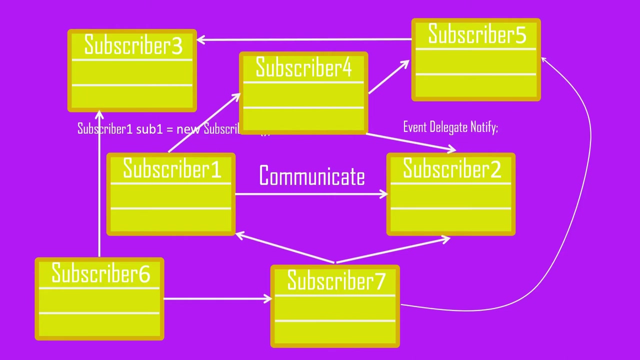 Okay, that's easy. We can either instantiate the object and communicate, Or maybe we can use an eventing mechanism. There could be other ways as well. But say, you have many such classes and they all wants to communicate with each other. In that case, I hope you realize how complex the reference maintenance would be. 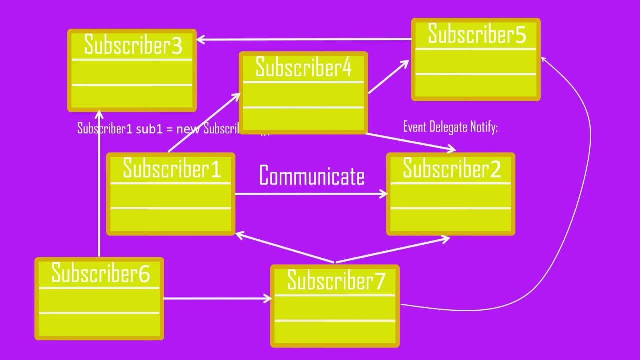 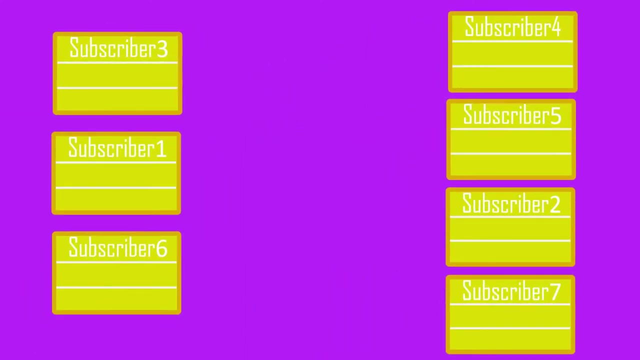 Perhaps each subscriber should maintain the reference of all other subscribers. That gives a very ugly, complex and difficult to maintain dependency graph. In this kind of situation the mediator pattern is best suited. Mediator Pattern allows object to avoid communicating directly. instead enables the communication. 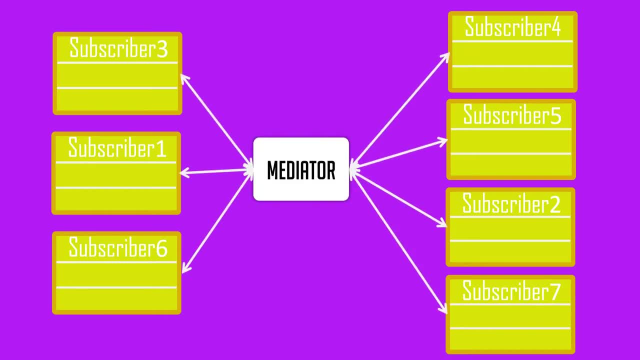 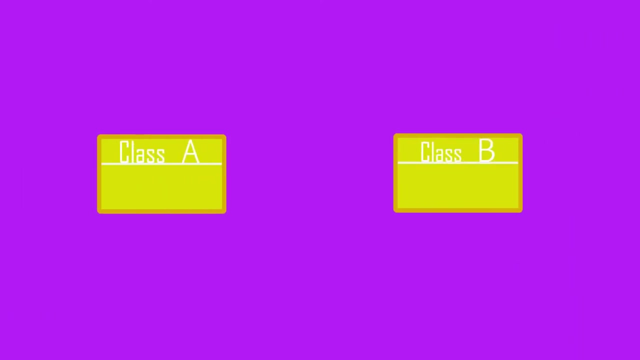 via central mediator. object: We will talk about some more specific points when we should implement this pattern, but for now let's see in detail all the components of this pattern and how this is implemented. 1. Let's say you have two classes. 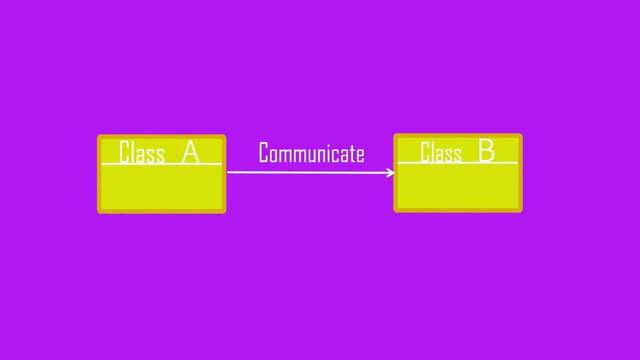 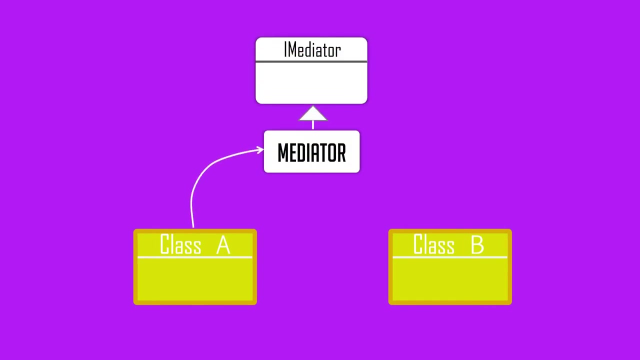 Class A and Class B that wants to interact with each other But, as mentioned, if we are using mediator pattern, then they will not interact like this. Instead, they will interact via mediator. Class A will call a method in mediator, something like method, publish and, in turn, mediator. 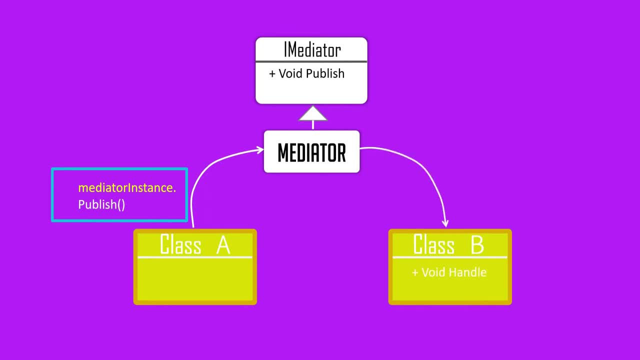 will notify all the classes who are interested to receive the message from Class A. Mediator will do this by again calling a method in Class B. I have named it here as method handle. Now to call a method of Class B, that's method handle. the mediator must have the instance. 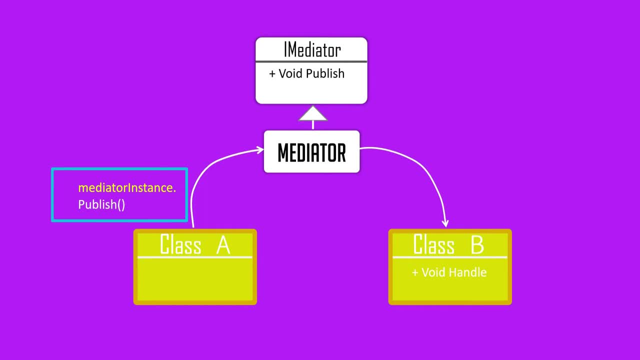 of B right. That's where each subscriber- I mean the classes- who wants to receive the messages from publishing class 2.. Let's make sure that their references are available in mediator. That's where we should have one more method in mediator. 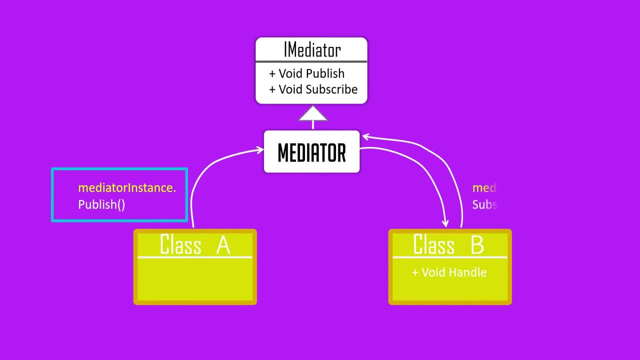 I call it as subscribe. This method is used by all the interested classes to add themselves to the mediator. You can see this here. That's the instance of subscriber sending it to mediator. It's a kind of bidirectional reference setting. Mediator has the instance of all the subscribers. 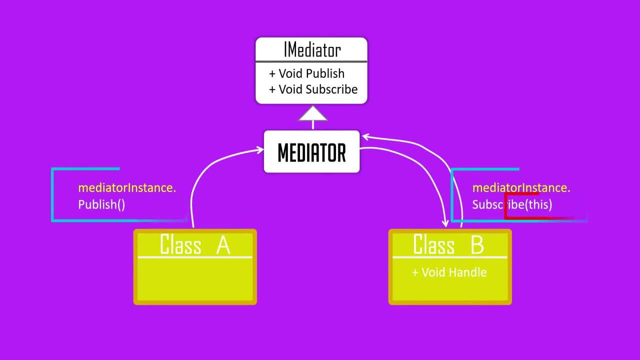 And subscriber has the instance of mediator. Now if there are one or two subscribers, then it is easy for mediator to keep those instances right. But as we know, there could be many subscribers, could be thousands. So mediator has to maintain all the subscribers in a list. 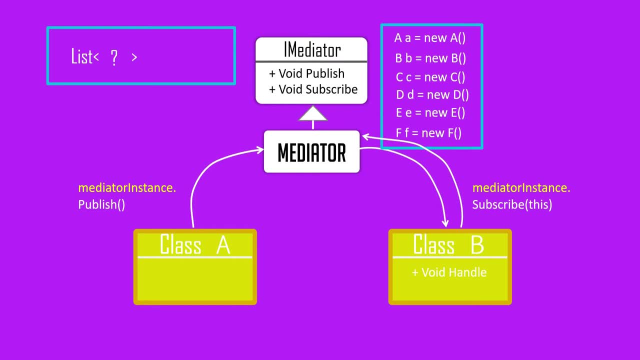 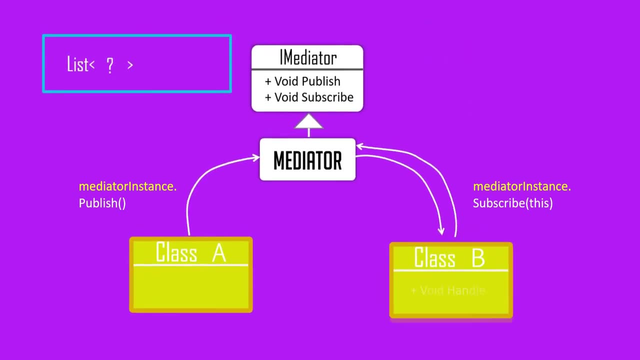 That's fine, But now the question is: what should be the type of the list, I mean what data type? That's where the pattern is. That's where the pattern is. So we can introduce one more interface for subscribers. I call it as isubscriber. 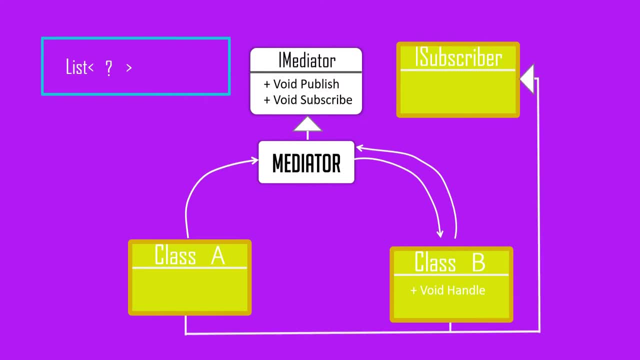 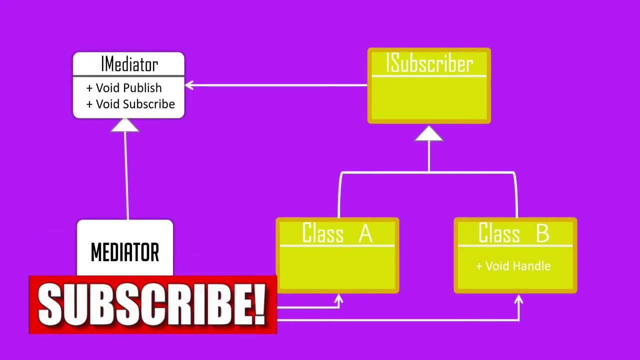 The interface must be implemented by all the subscriber classes. And now mediator can safely maintain a list of isubscriber, which will be nothing but list of all the subscribers. Now, if we rearrange the diagram, then we get the UML that we have seen in the beginning. 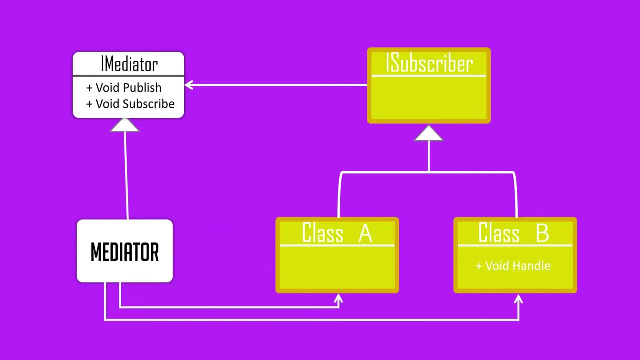 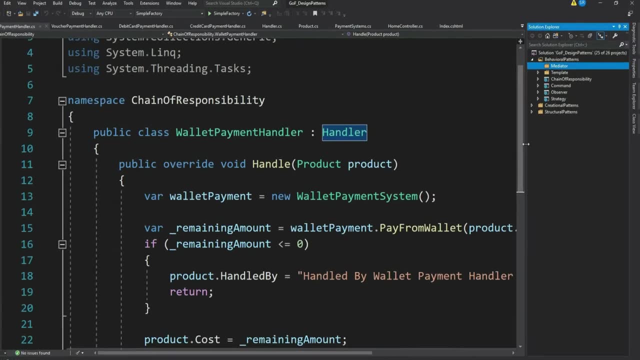 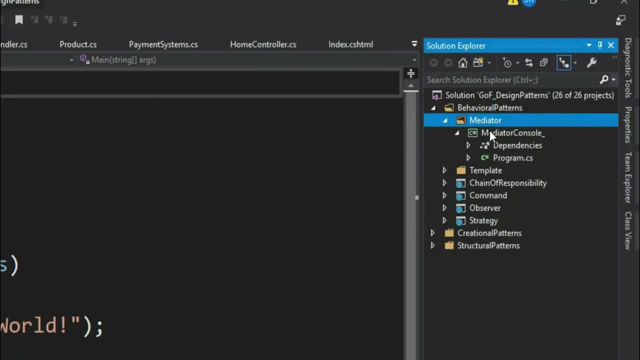 I hope you have some idea now how mediator pattern works Before we go through when exactly we should use this pattern. let's implement this in a console application. So let me create a console application. Let's create a folder called subscriber. Here I will create all the classes that wants to send and receive messages. 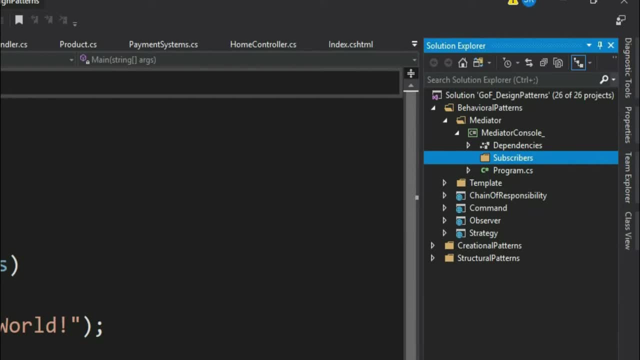 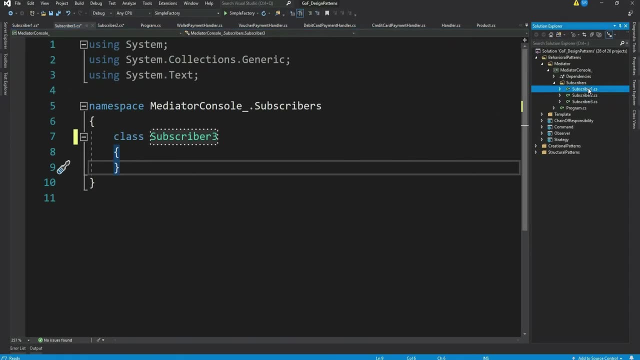 I mean the classes that wants to interact with each other. Let me create those classes. first Let's create a folder called subscriber. Here I will create all the classes that wants to send and receive messages. So I have three classes here: Subscriber 1, 2 and 3.. 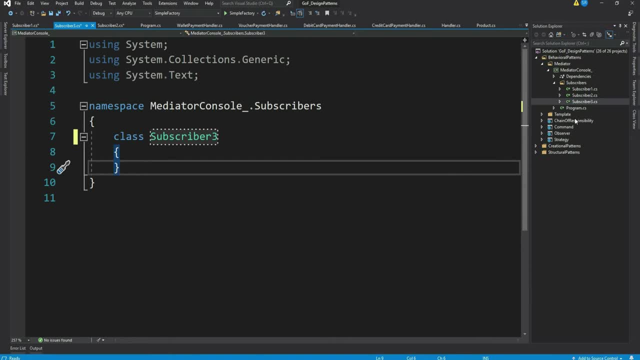 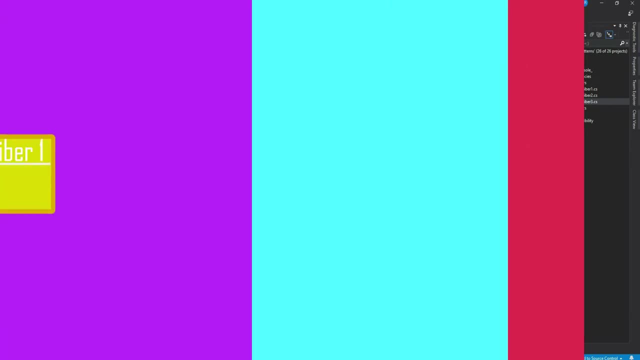 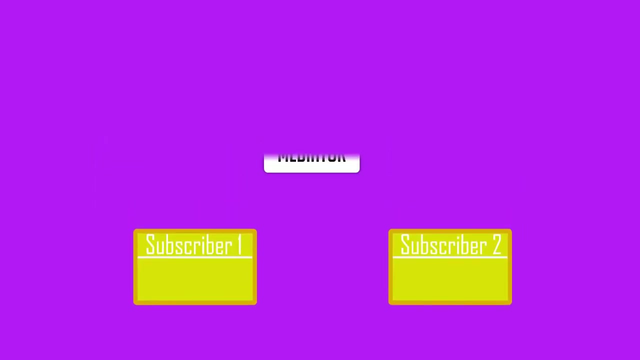 I will not write any business logic here. Let's assume that it does lot of things for now May be read, write to database or something else, And now it wants to send some messages to each other. But remember, it does not want to interact directly. 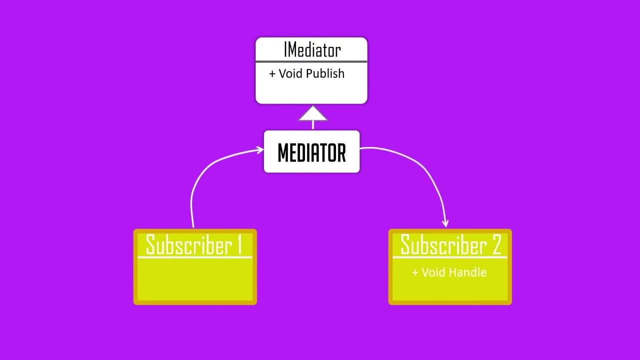 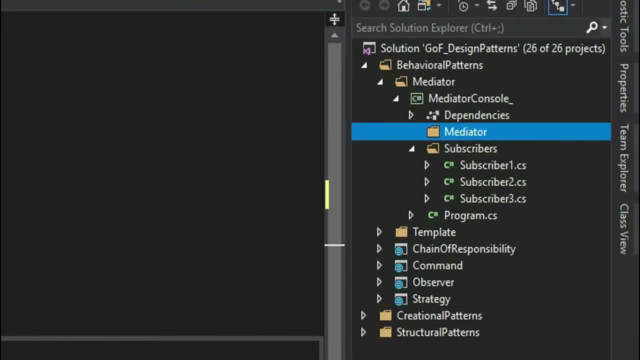 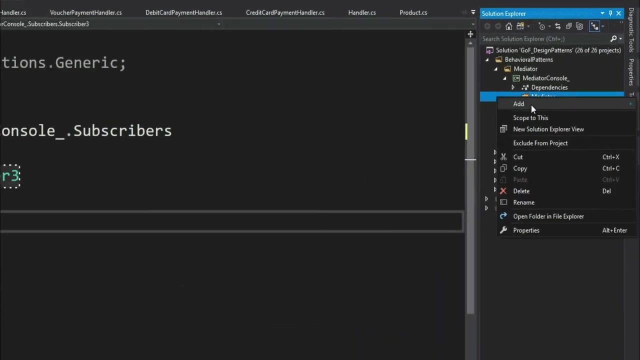 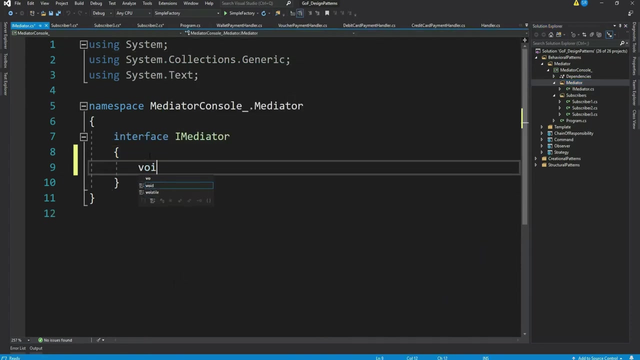 Instead via a mediator. So let's create another folder mediator. I will keep all the mediator related classes and interfaces here. Let's first create our mediator interface imediator What it will have As discussed: a publish method. This method will be called by the object that wants to send messages. 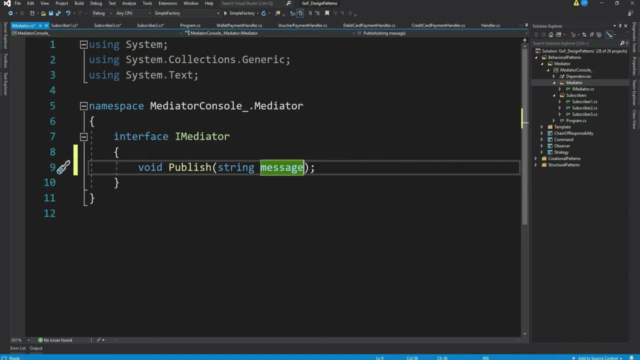 In our case, may be some of the subscriber who wants to publish message. Please do note that implementations of mediator pattern may have some variations. This is a very simple implementation, just to understand the pattern for now. Right now it can just handle a single string message. 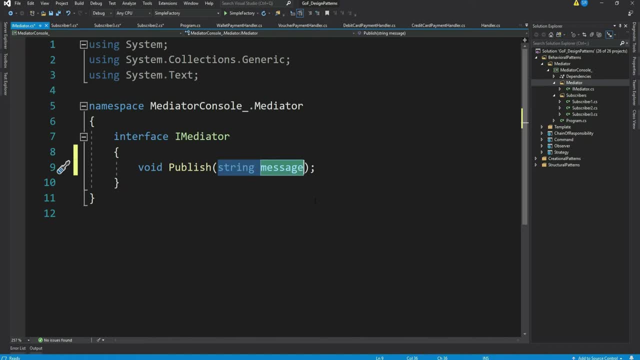 But in real time application you have to handle different types of messages and also have to ensure that it is received by only the interested subscriber. Let's see how it works. And to handle different types of messages, the implementation would be a bit complex. 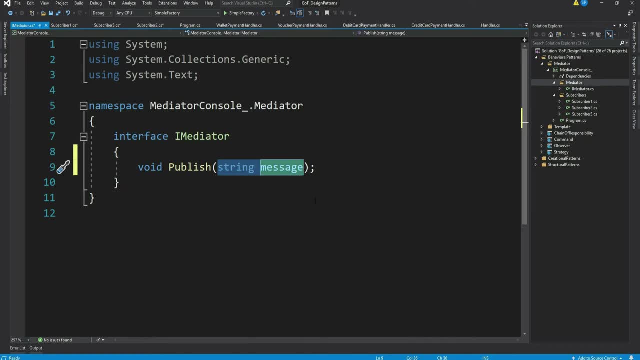 I will show you that when we will implement this pattern in WPF MVVM application. For now, let's complete this interface implementation, So we should have one more method here, right: Subscribe. This method will be called by all the subscribers to add themselves to the mediator. 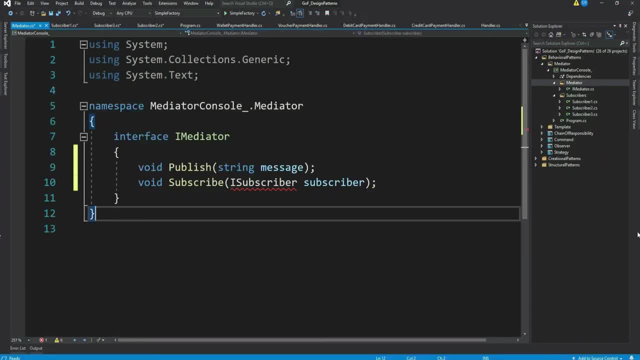 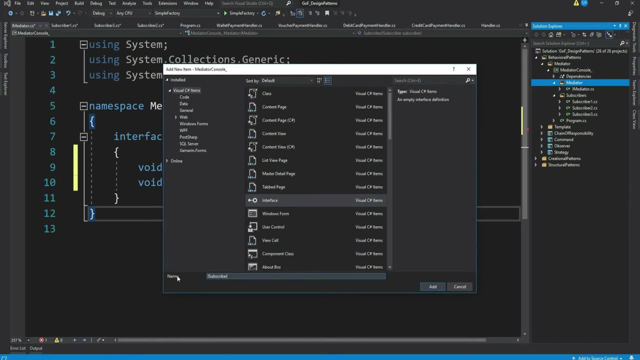 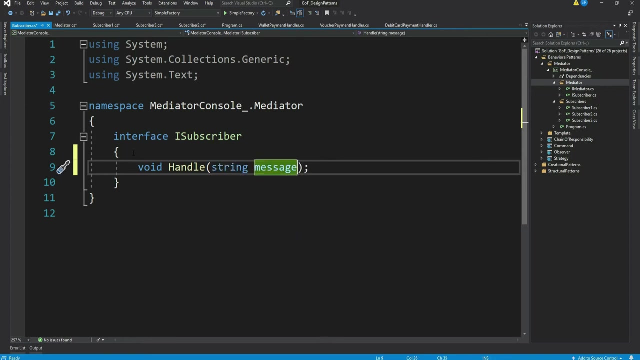 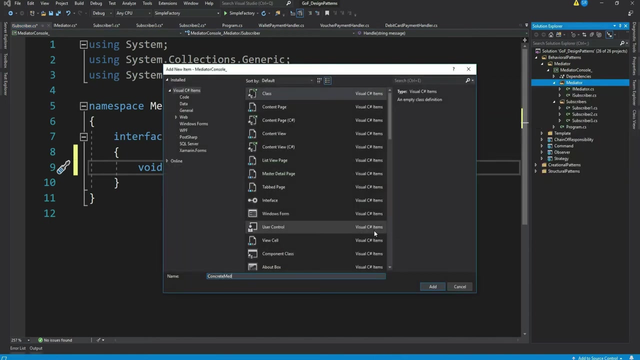 iSubscribers are the object: who are interested in receiving messages. Let's create iSubscriber interface. It has a single method handle. This will be invoked by our mediator. Now let's create our concrete mediator. Let's implement iMediator. Let's create iMediator. 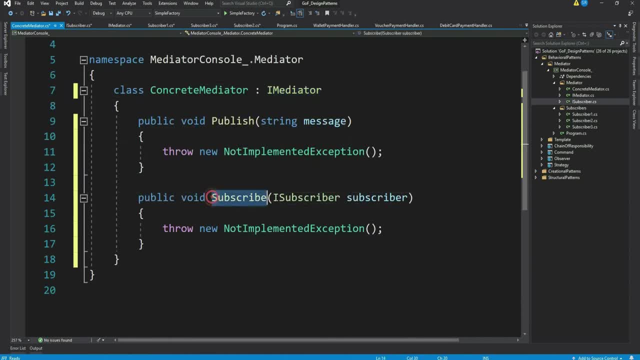 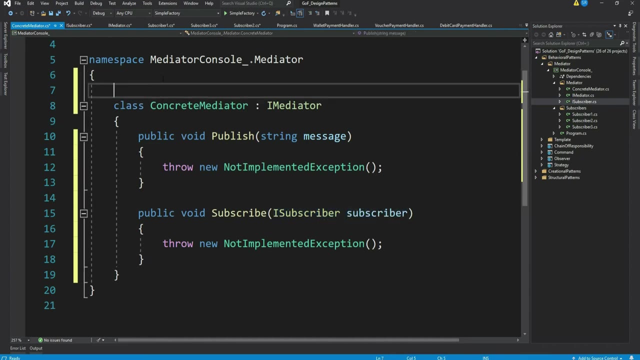 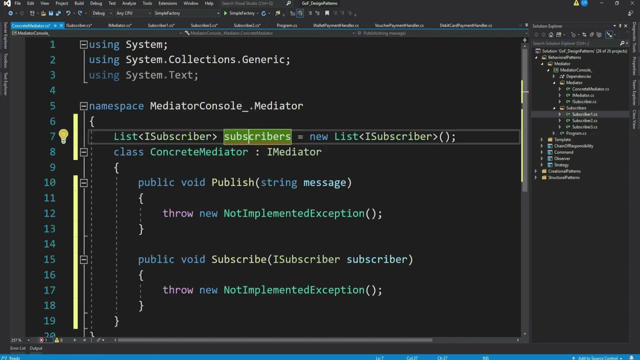 Let's create iMediator, So this subscribe method will receive all the subscribers whenever subscriber subscribes themselves. And to maintain all the subscribers here. what do we need? Yes, we need a collection. Let's create a list Now. let's add the incoming subscriber to the list. 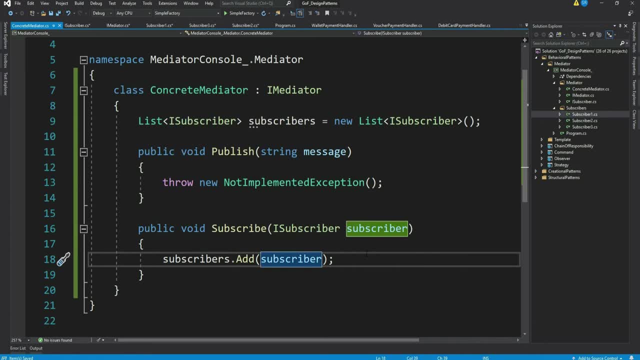 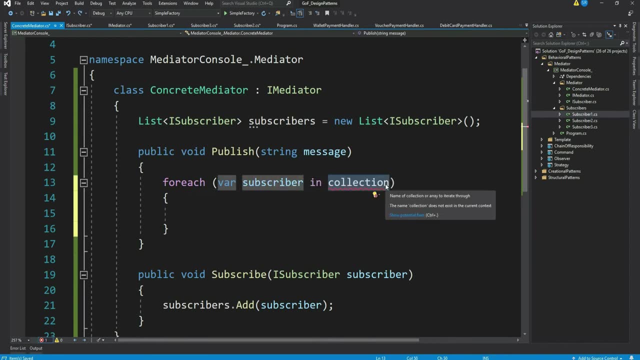 Let's create a list. Ok, what publish method should do? Yes, it should loop through all the subscribers in the list And call handle method. Now this handle method will be there in all the concrete subscribers. Let's implement our iSubscriber interface to our subscribers. 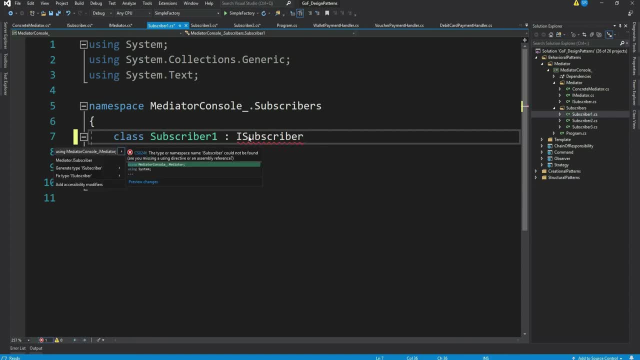 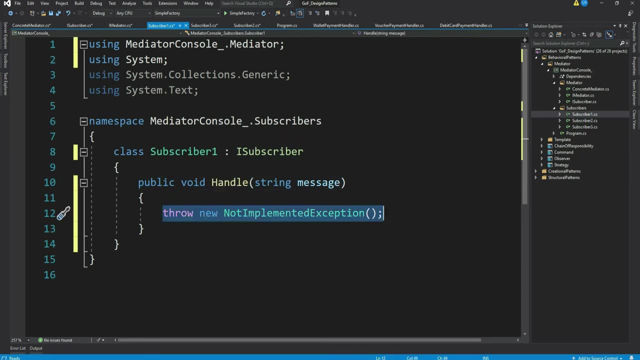 Ok, Let's create a list. Ok, And to change it, We will add our iSubscriber here And we will add our iSubscriber CSS. We will enter our iSubscriber in here And we will add our iSubscriber here And we will enter our iSubscriber in here. 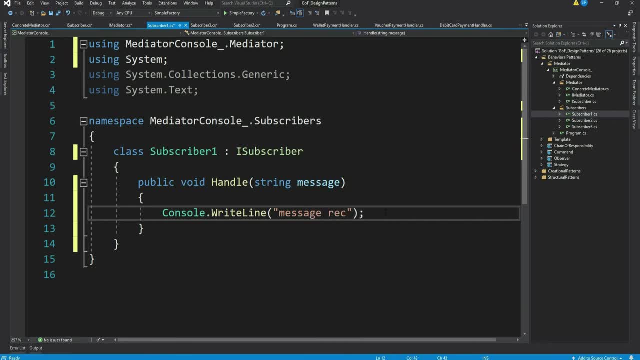 So we have the method handle here. For now, let's just print a simple message Message received by subscriber 1. Let's do the similar kind of implementation to other subscribers. So our subscriber implementation is done, Or is it really done? 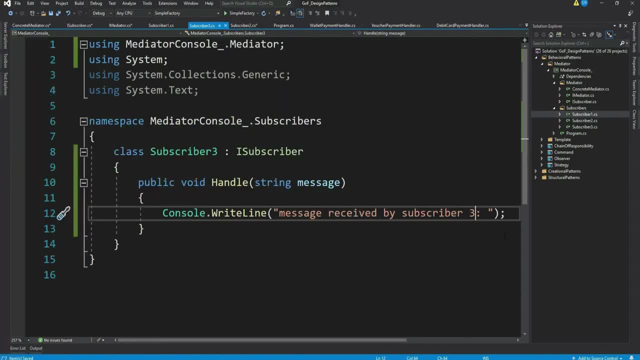 Are we missing something here? Well, let's go ahead and add a new subscriber to our iSubscriber And we can open one of the iSubscriber for our iSubscriber. So our iSubscriber implementation is done, So our iSubscriber is now back. 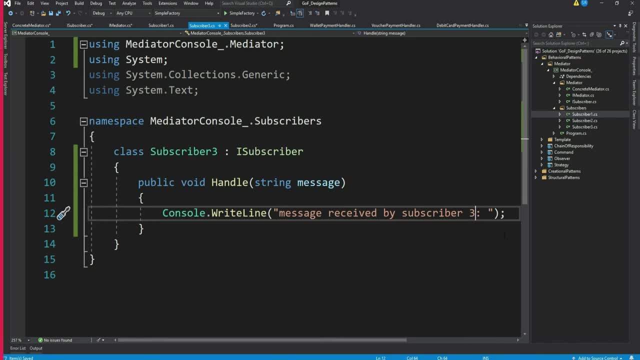 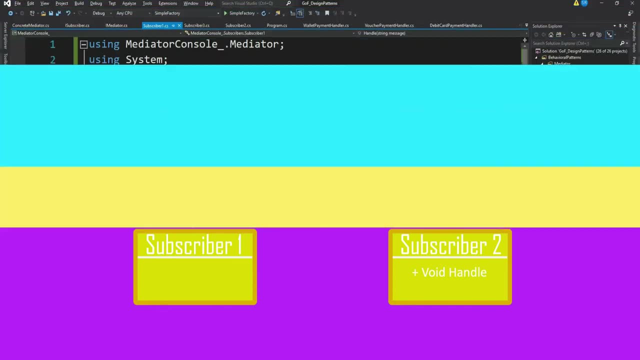 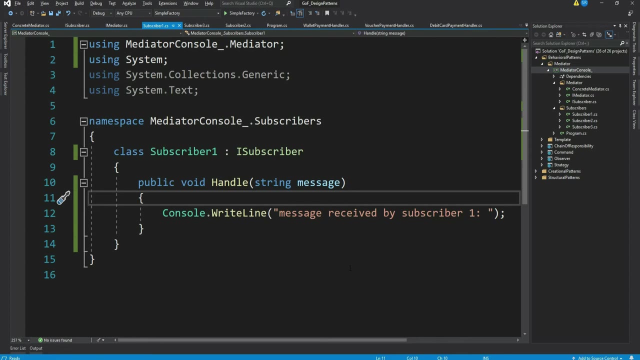 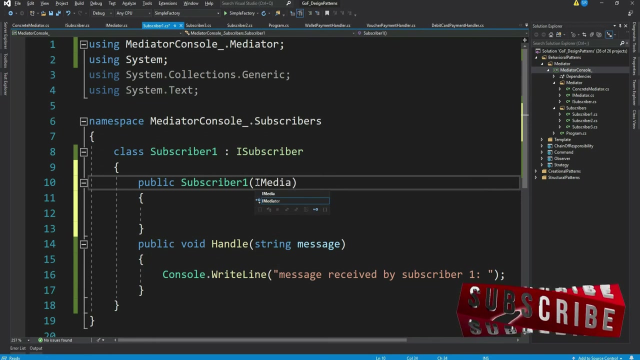 are we missing something here? yes, definitely missing right. remember, we have to add our subscriber to the mediator, and for that we have to call a method in mediator, and hence we need mediator instance here. so let's inject it via constructor and call subscribe with this instance, so with this. 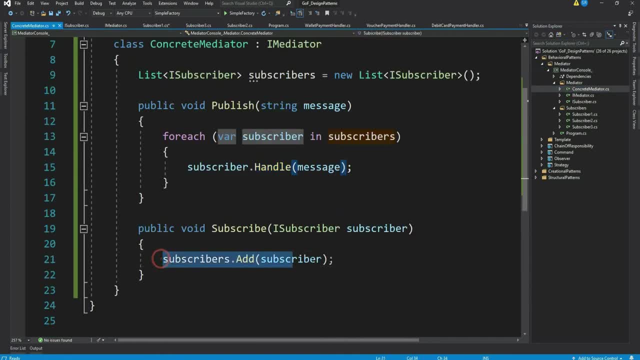 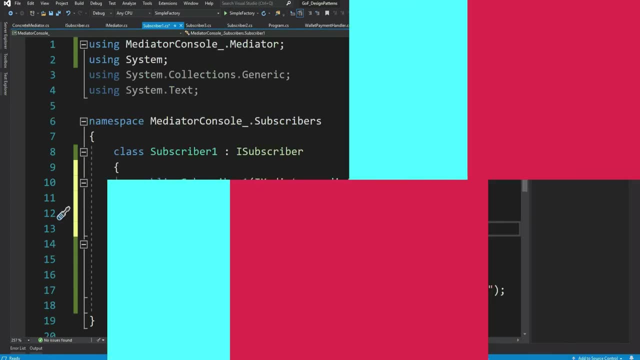 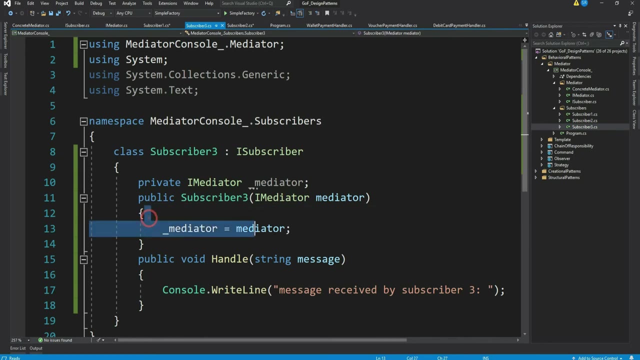 statement mediator adds this class instance to its list. okay, now let's do the similar implementation again with other subscribers as well. so here we are subscribing this as well, for the message suggests. but if you see subscriber 3, we are not subscribing here what it means. it means this class is not interested to receive messages, or we can say that when 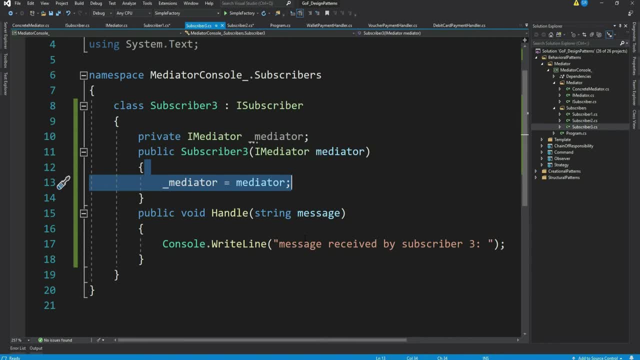 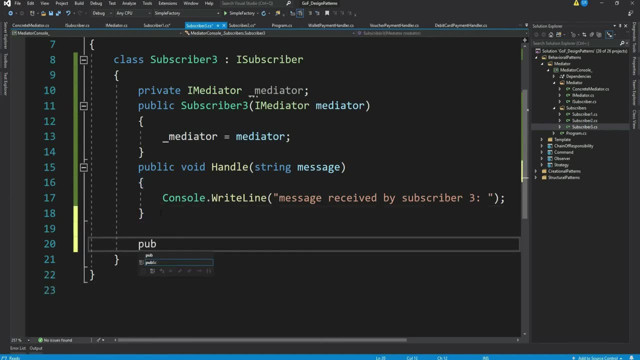 someone publishes a message, this class will not get any notification. let's say, this class wants to publish the message, so let's create a public method here. let's publish a message. how do we do that? yes, using mediator instance. I hope you are able to relate to what we have discussed earlier. 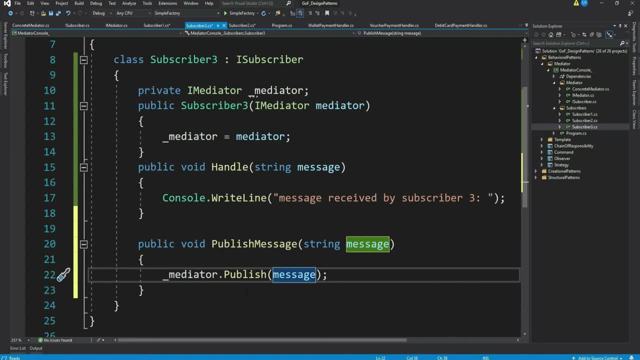 this class basically publishes some messages which are received by subscriber one and two, but for this interaction, the publisher class do not directly call the receiving classes. instead it also will call the receiving classes and in this case you will be getting messages to mediator and mediator will in. 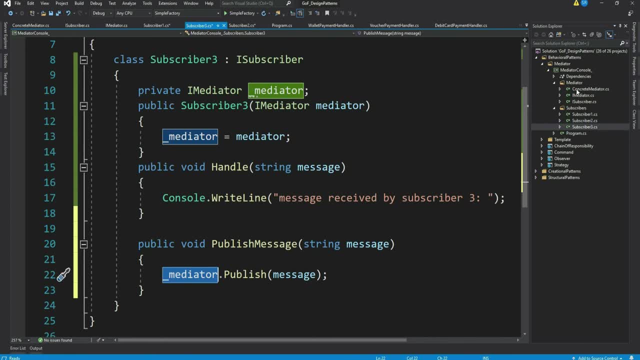 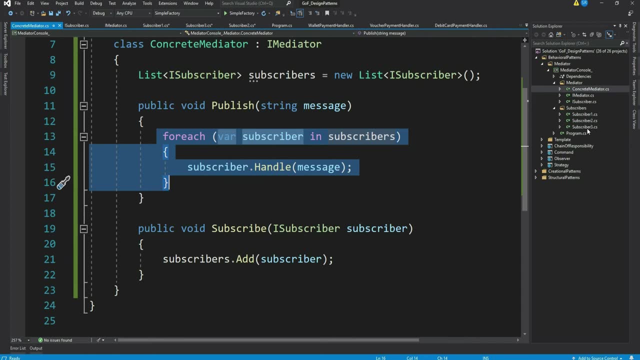 turn, send it to all the subscribers. the only prominent flow in this implementation is that right now, mediator will send the messages to all the subscribers in its list. I mean, with the current implementation we cannot send the message to only selected subscribers. but, as mentioned, I will show you that in just a bit. 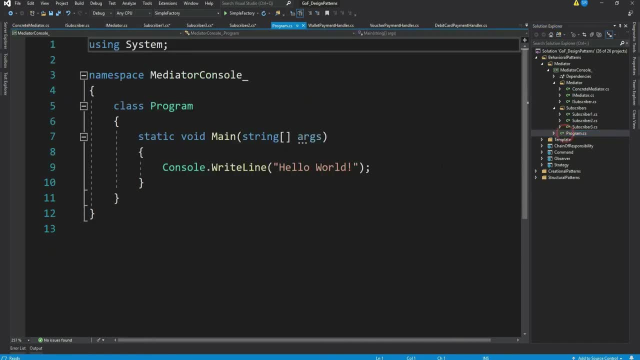 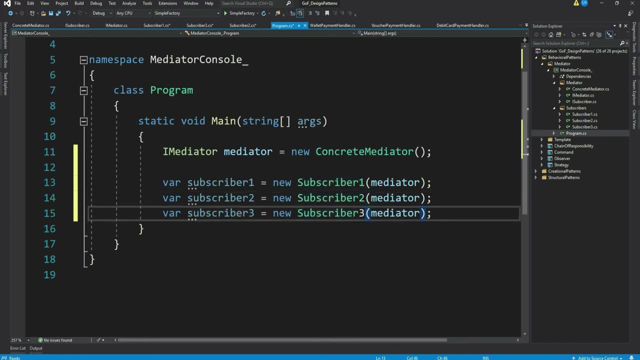 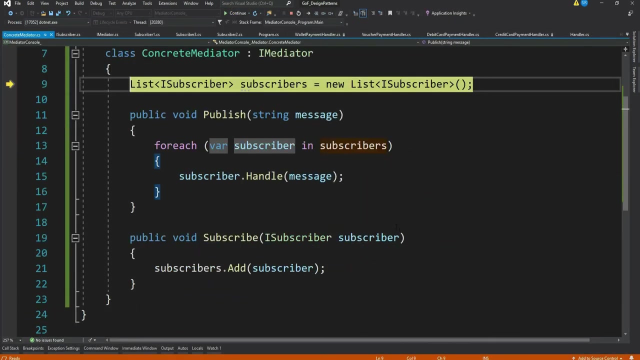 this all up from our programcs class. Let's instantiate our mediator. Let's instantiate our subscribers as well and pass mediator instance to it, So our subscriber instantiation is done. Now let's publish a message from subscriber 3 class. Let's put a breakpoint and debug this So it instantiates mediator, and then 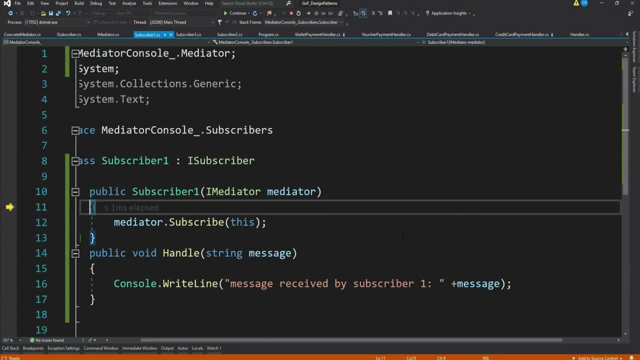 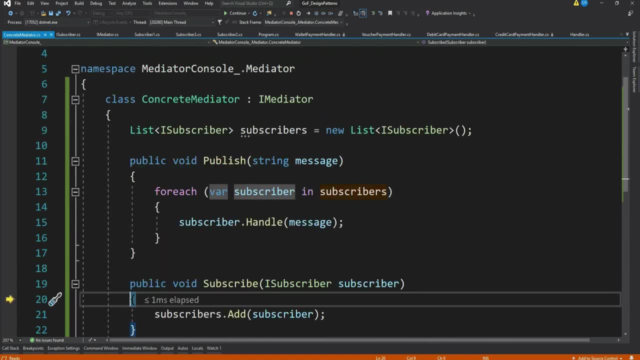 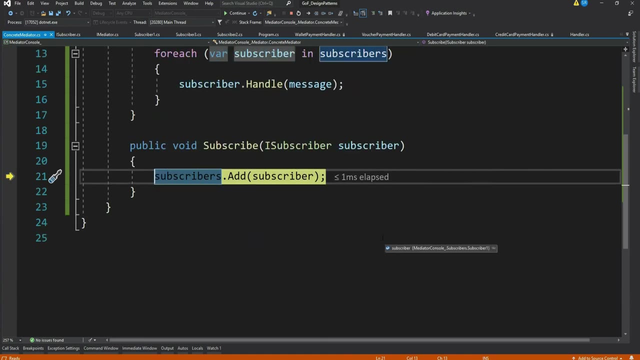 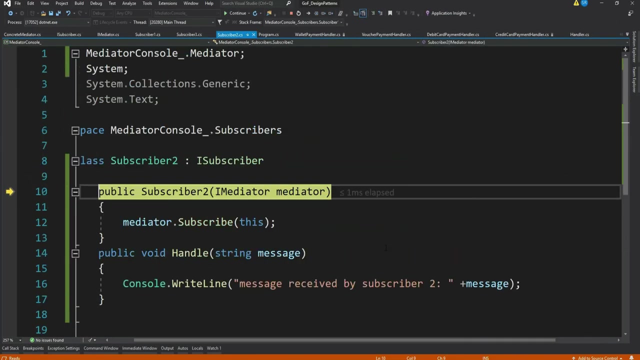 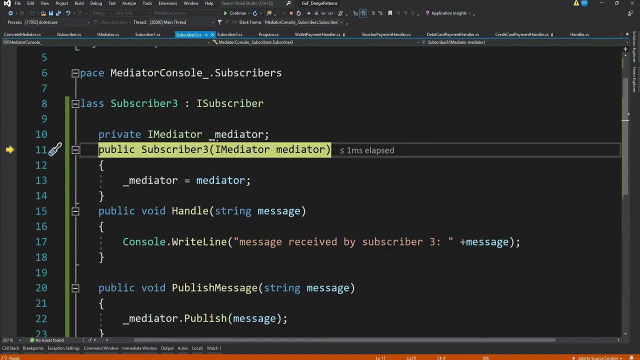 subscriber 1.. Subscriber 1 receives the mediator instance and subscribes itself. So it goes to ConcreteMediator class and adds the subscriber to its list. See: the subscriber is subscriber1.. It comes out Again. does the same thing for subscriber 2 as well and for subscriber 3, just. 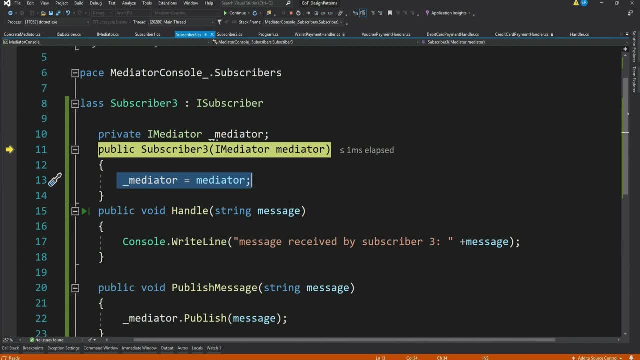 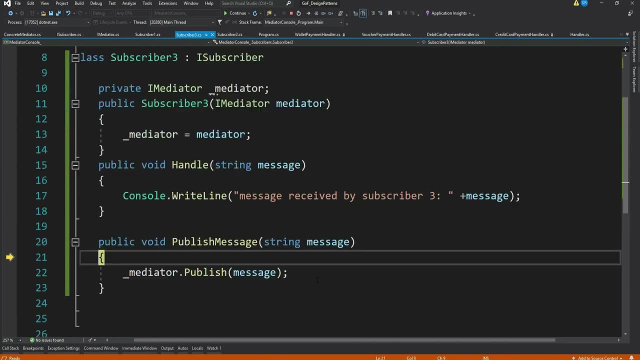 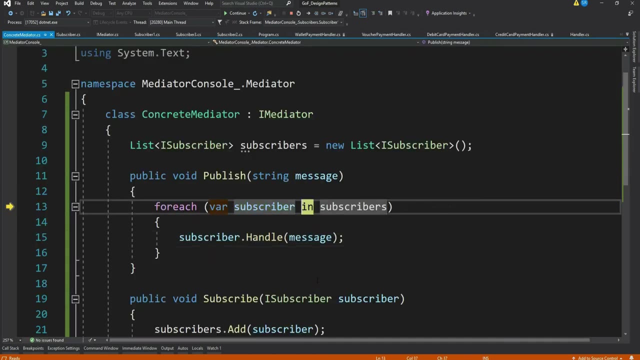 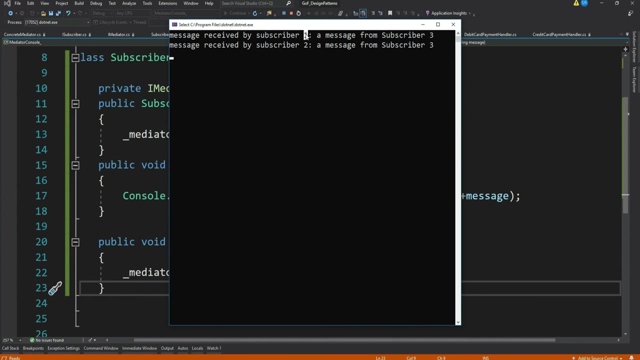 stores the mediator instance to a class level variable. that's because we want to use this down here now. it calls the publish method, goes to mediator loops, through the subscriber list, goes to respective subscriber handle method and we get the expected result. subscriber one and two receives the message. 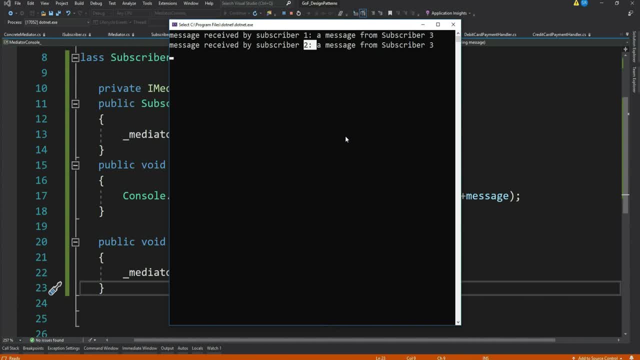 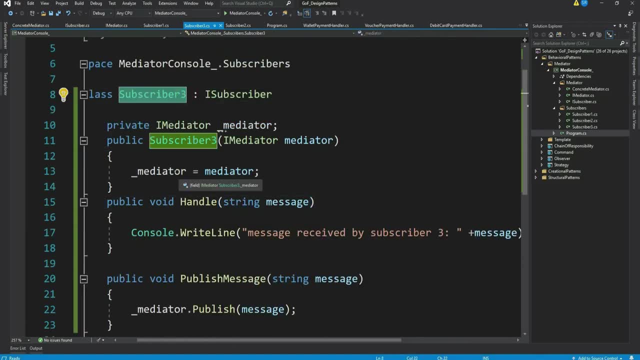 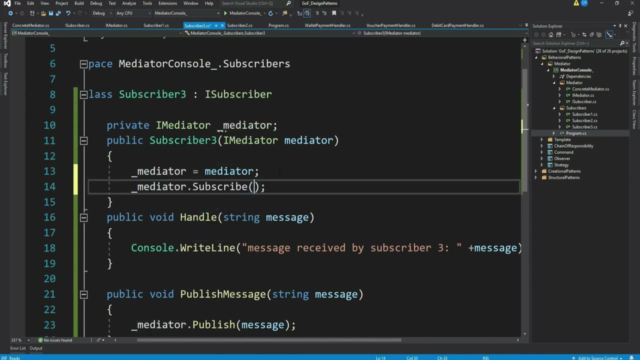 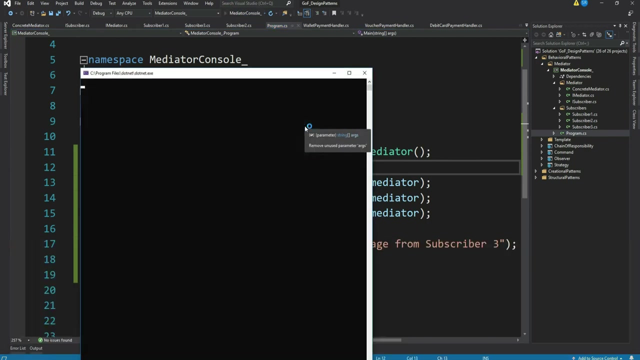 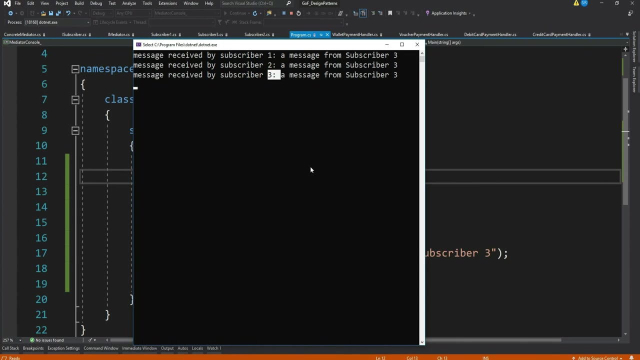 but not subscriber three. now say: subscriber three is also interested in its own message. so what we are required to do? just subscribe for the message. let's do that, let's run it and see. now see, subscriber 3 also receives the message. now say: subscriber 2 is not interested. so what should we do? just remove the subscription. 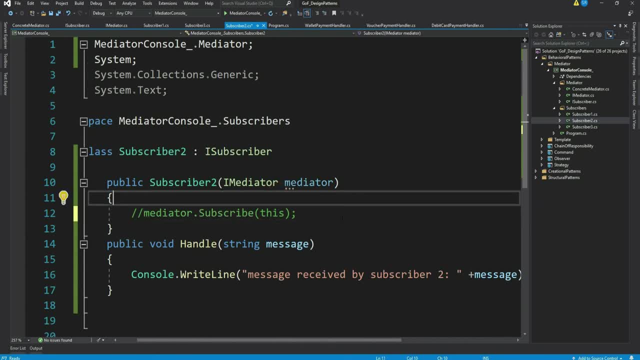 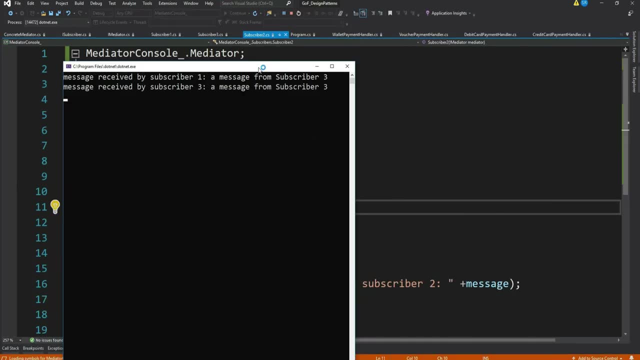 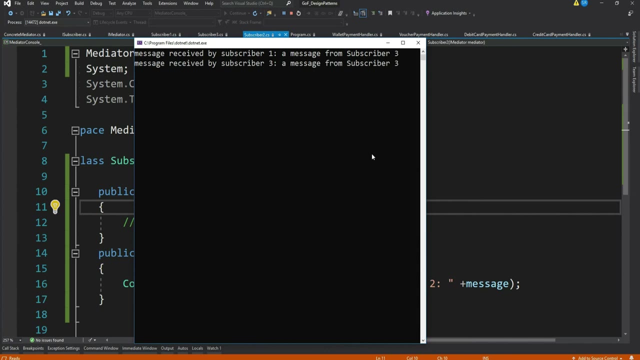 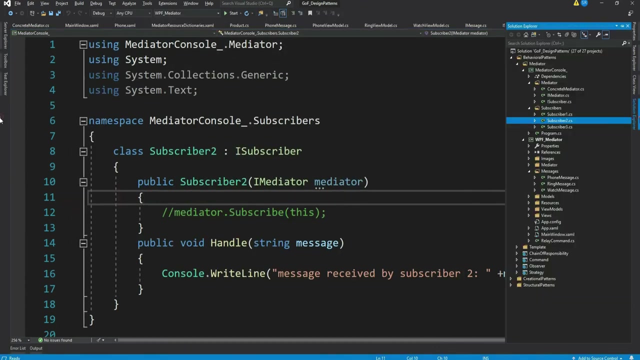 note that ideally we should have a method in mediator to remove the subscriptions. let's run it. see, subscriber 2 does not receives the message now. okay, with this, we are done with our simple console implementation of mediator pattern. I hope it was simple. You have to implement this mediator class once and you can use this in your entire application. 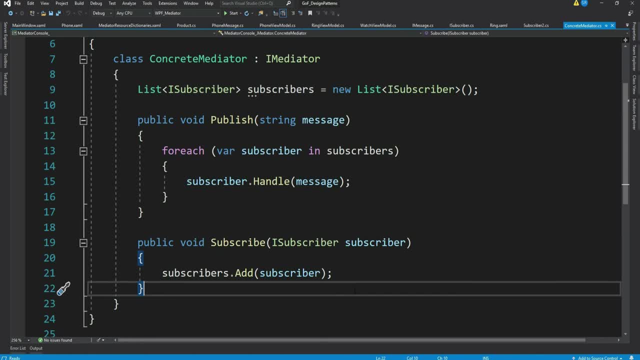 for sending and receiving notifications with the required message. But, as mentioned earlier, there are few prominent improvement areas in this code. As you have seen, this implementation just loops through the subscriber list and sends only one type of message. In our case, that's a string. 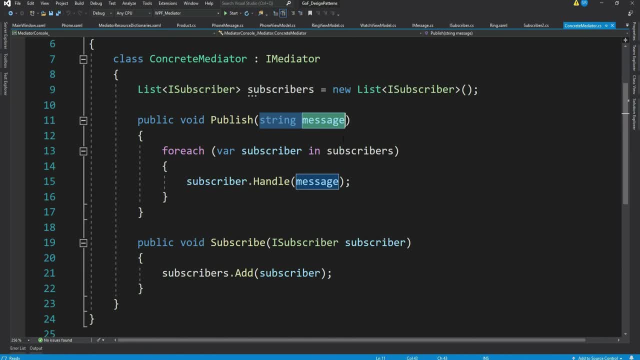 But how about sending different types of domain messages like product, product order or customer information? I mean messages based on business requirement. That's not possible. This code is not generic enough to handle that. I have created a second part of this video where I have used a WPF MVVM application to 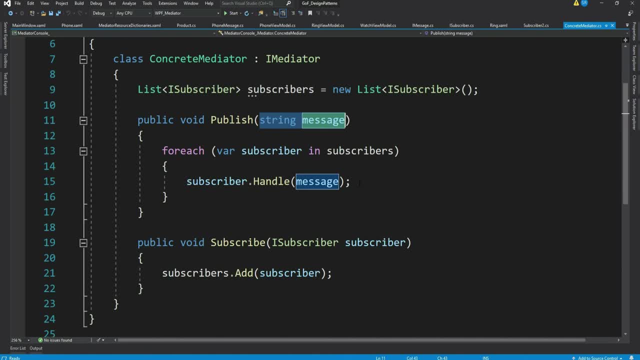 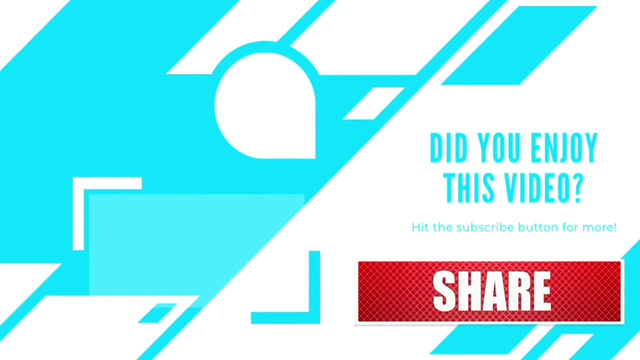 demonstrate how exactly this pattern is implemented in a real-time application. Don't miss to check out that. Let me end this part here. If the content was helpful, don't forget to subscribe the channel and drop in comment for all the future videos on C sharp and other technologies. Thanks. 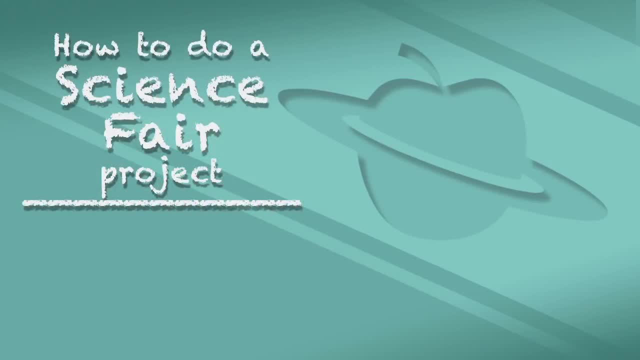 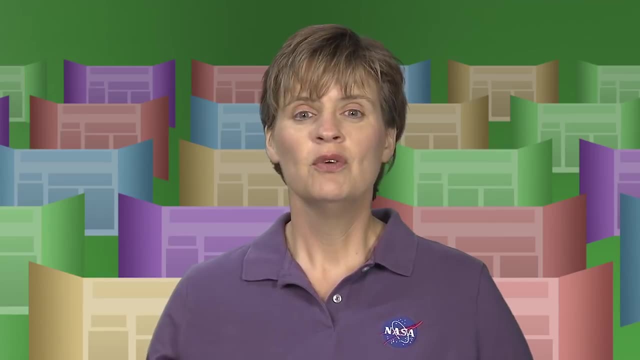 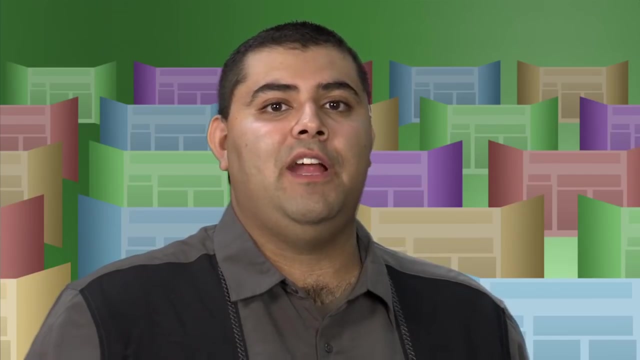 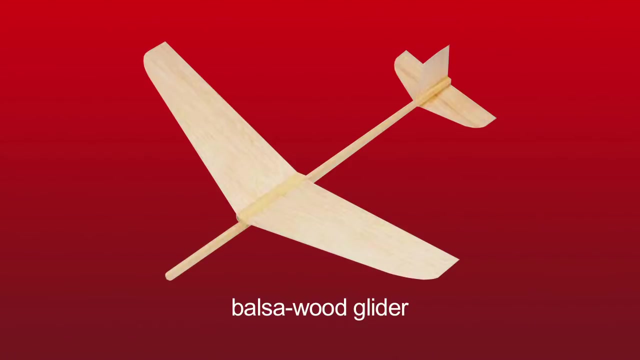 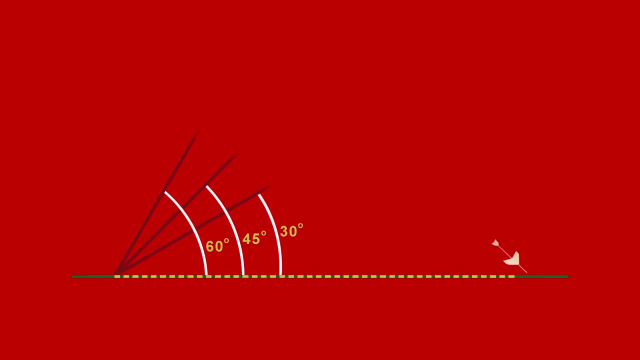 Now it's time to design your procedure. Remember: you're only changing one variable and you need to conduct your experiment multiple times for each trial. Each trial needs to be repeated in exactly the same manner. Let's look at the airplane for procedures. Instead of an airplane, let's look at a BOLSA glider. You try to keep everything constant, except for one variable. In this case, let's look at the angle of launch, Launch it at different angles and measure the distance it covers. You have the same glider for every experiment. You try to keep the launch force constant throughout the experiments And for each angle, you throw it multiple times, So you get several data points at each angle. Once you do that, you repeat the steps.